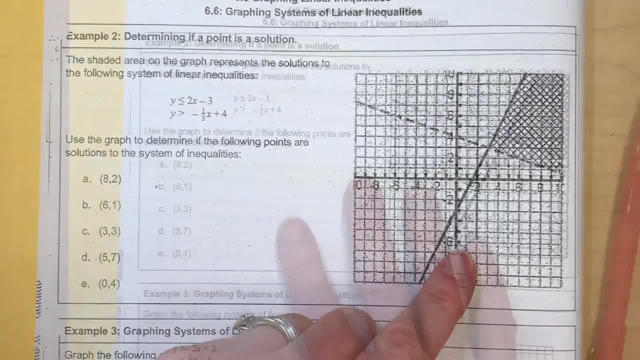 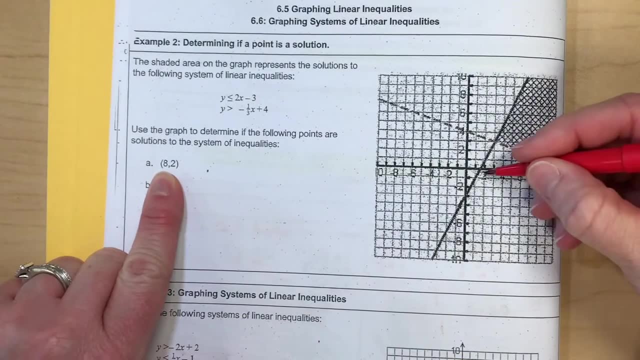 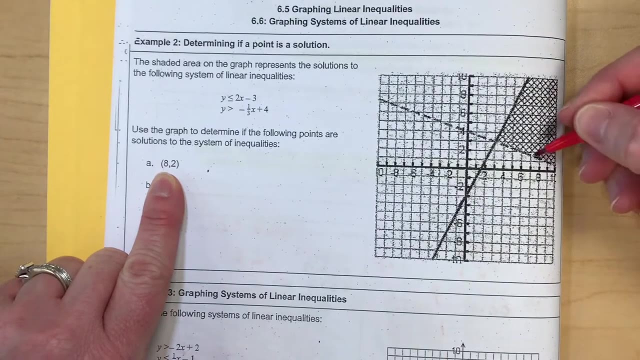 The first point is 8, 2.. Hold on one second. Thanks for letting me take a break to answer that phone call. All right, so 8, 2.. This point would be 2, 4, 6,, 8, up, 2.. For sure that is inside your shaded region, It's not on your. 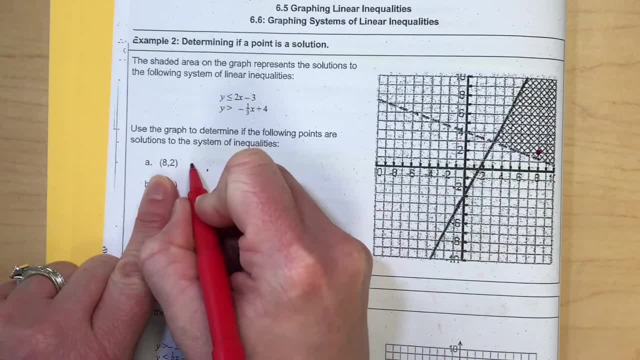 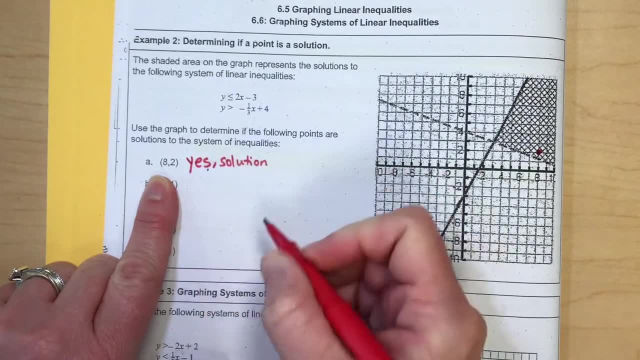 dashed line. So this would be a solution to your system. So I'm actually going to write: instead of true or false, I'm going to write yes or no. Yes solution. Okay, now our next point, 6, comma. 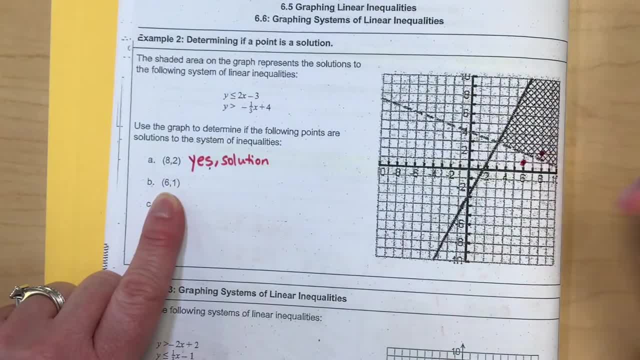 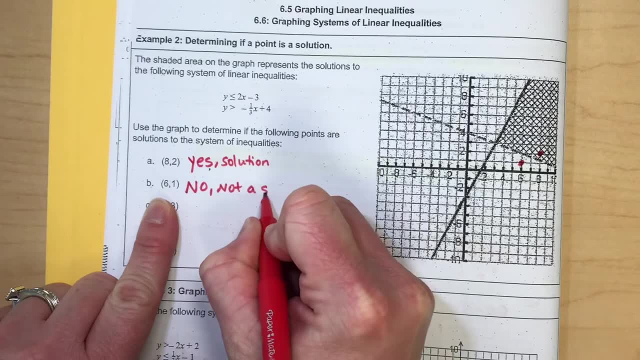 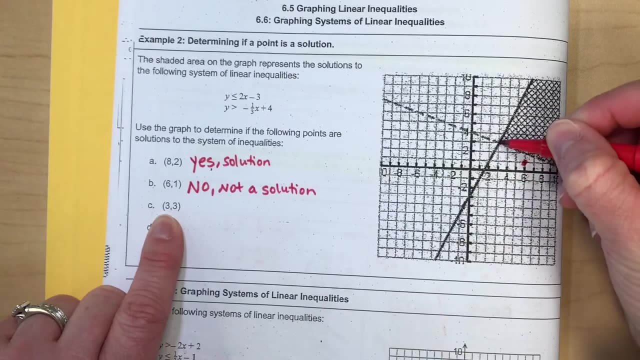 1.. 2, 4, 6, up. 1. This is not in the shaded region, It's not on a solid line. So no, this would not be a solution. Okay, number 3, 3.. So 1, 2, 3, up. 1, 2, 3.. Now an intersection, that is, with your system. 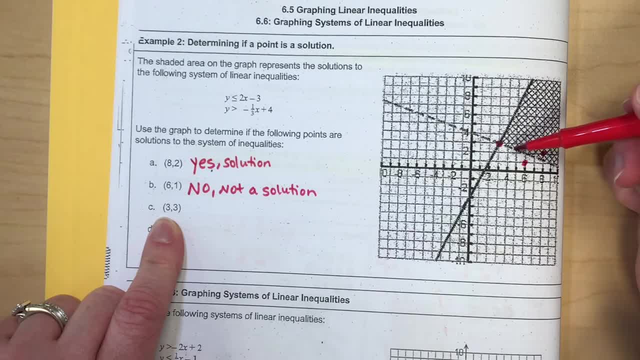 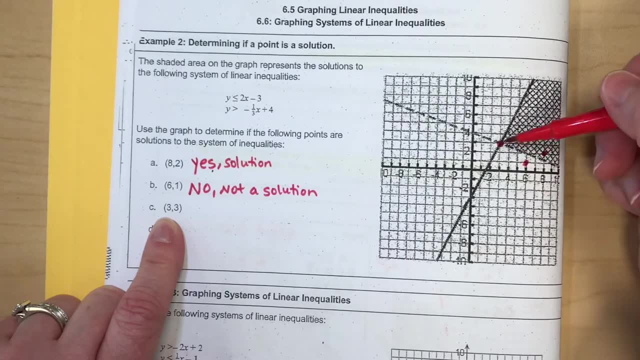 if it touches a solid line and a dashed line. So let's think about this. At first reaction, my gut would be like: oh yeah, yeah, that touches a solid line, It's good, But this is a system of equations And it has to work for both of them. So if it touches a solid line and a dashed line, 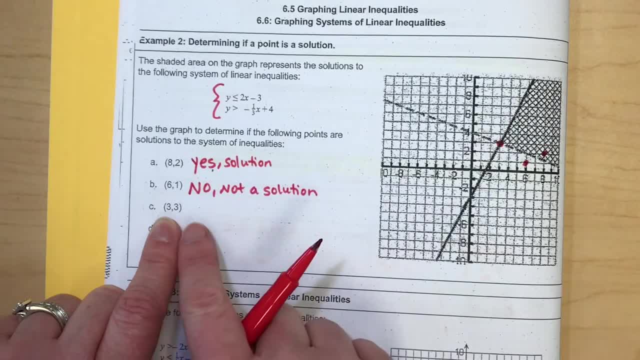 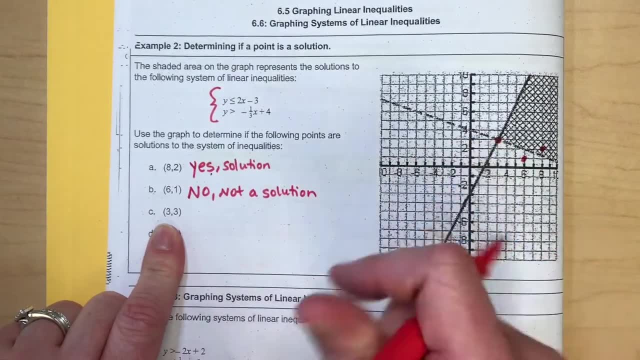 for it to be a solution to the system, And so let me give you like a really weird real life example of this real quick. So here's your answer for this: And it's no, and I'll explain why. Not a solution. 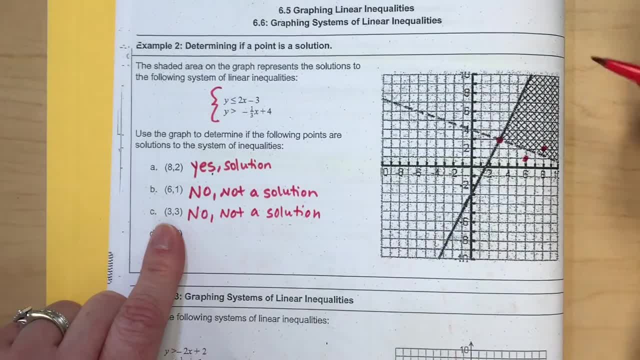 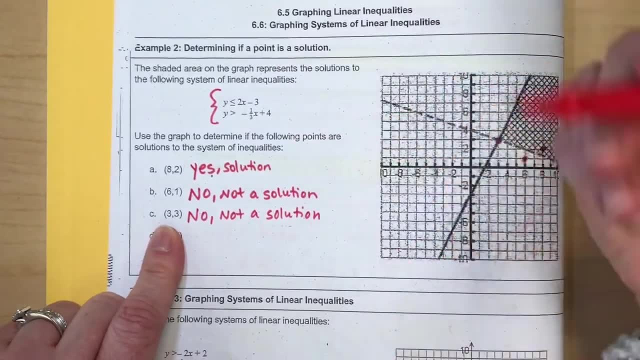 I recently learned that I have grown into an allergy to tree nuts, And so, talking about solution to a system in my household, my husband and I have agreed that we don't have the tree nuts in our home because it would be a problem, And so I'm going to give you an example of a system, And so I'm. 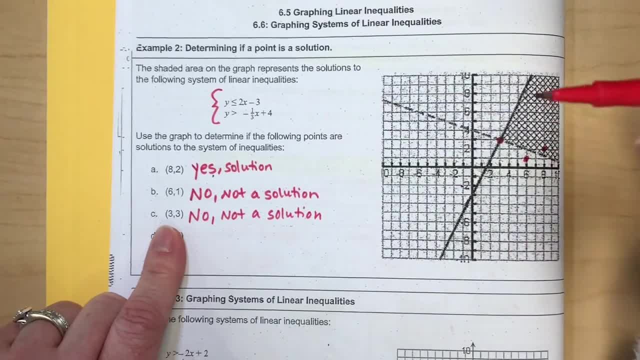 going to give you an example of a system, And so, talking about solution to a system in my household, My husband and I have agreed that we don't have the tree nuts in our home because it would be, let's say, deadly to me, because if I somehow, you know, have the tree nuts or I'm, you know, moving. 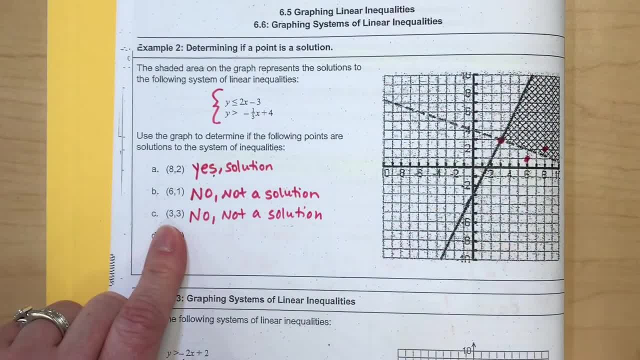 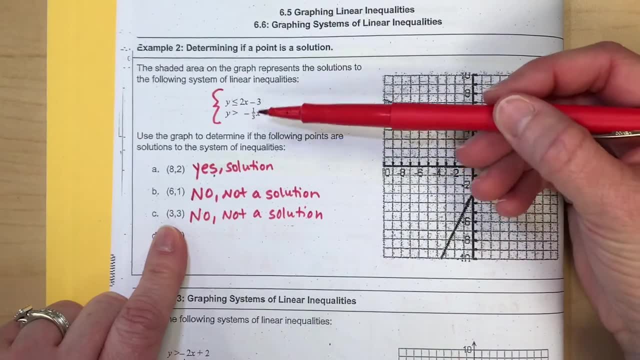 stuff around and I was touching them. and then let's say, I touch my eyeball or, you know, my mouth. that could be very dangerous for me and so if it doesn't work for both systems, it doesn't work for the system, meaning no, it's not a solution. so the reason why no here is because if you're dealing